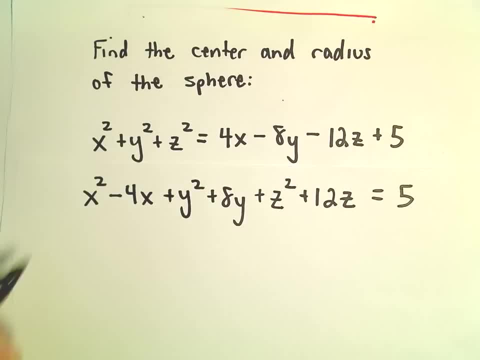 And I'm going to leave the constant 5 on the right side. So now to do the completing the square term. I'm going to give myself a little bit of room. Hopefully you've seen completing the square. It's one of these things. 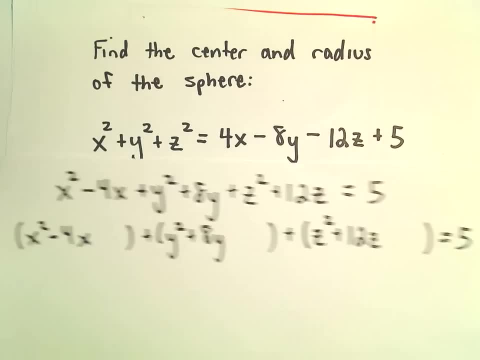 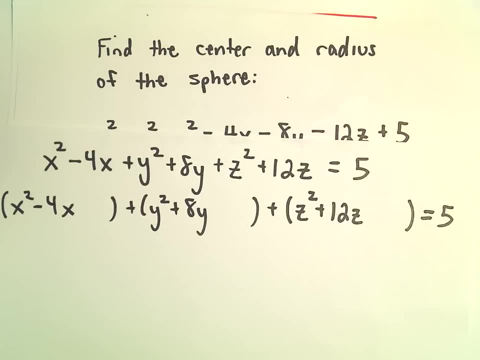 You use it a little bit, not terribly often. You use it, in fact, to integrate some functions you have to use completing the square. So again, the idea is: let's see if I can fit it all in here. I'm going to take the coefficient in front of x, which is just negative 4.. 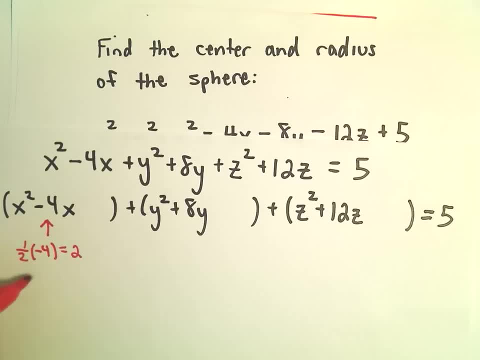 Again, I take one-half of that coefficient. that's going to give me positive 2.. I square it, which is going to give me a 4, and I just throw a plus 4 in the parenthesis. I go to the same thing. I look at my 8y. I take one-half of the coefficient on the y. 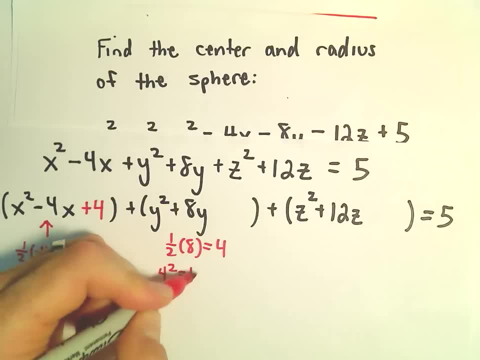 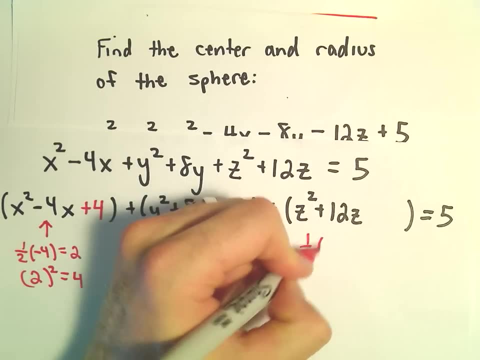 So one-half of 8 is going to be 4, 4 squared is going to be 16, I plug a plus 16 in there out of nowhere, And same thing I'll do one-half of 12, that'll give me 6.. 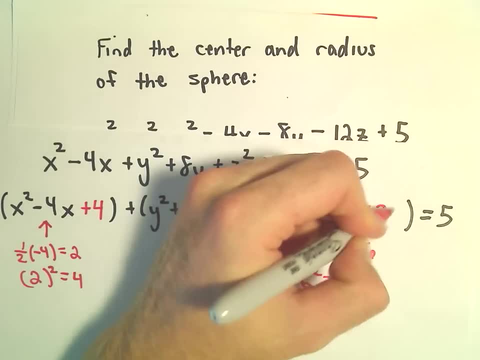 6 squared is going to be 4.. 6 squared is going to be 4.. 6 squared is going to be 4.. 6 squared is going to be 36, so I'm going to add 36 into that set of parentheses. 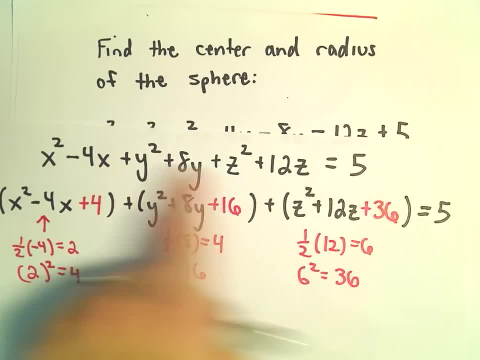 So now we have to be careful. you know, if you undid the parentheses, everything would be there, but we would have extra things. Namely, we would have an extra plus 4,, plus 16, and plus 36.. 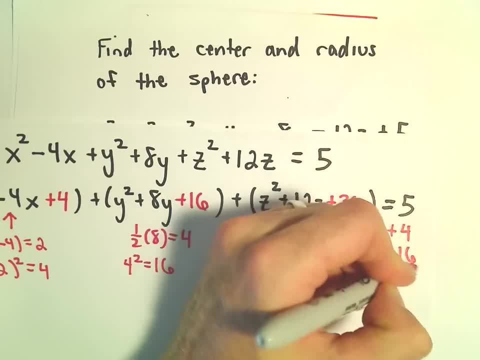 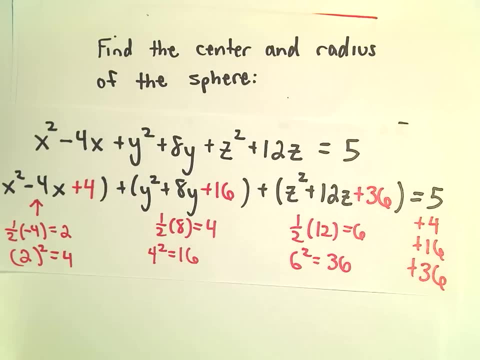 So, on the right side, I would have to add 4, and I would have to add 16, and I would have to add 36.. So I'm going to make sure that I do that as well. So I'm going to make sure that I do that as well. 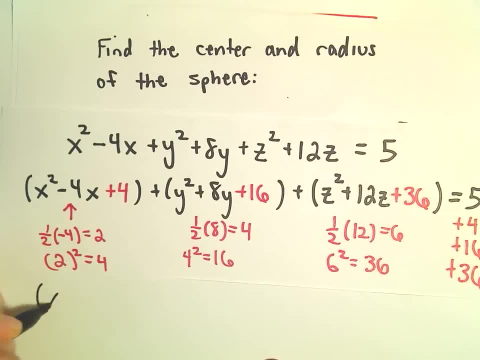 So now the idea is: x squared minus 4x plus 4 is a perfect square. We can simply write that as x minus 2, quantity squared y squared plus 8y plus 16,. we can write that as y plus 4 squared. 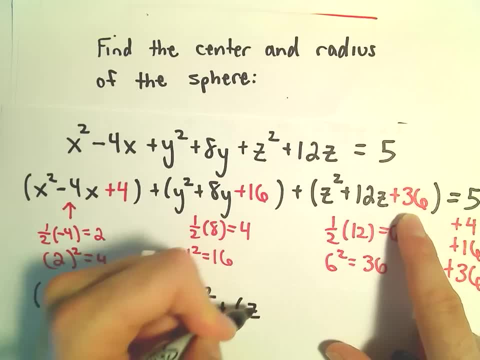 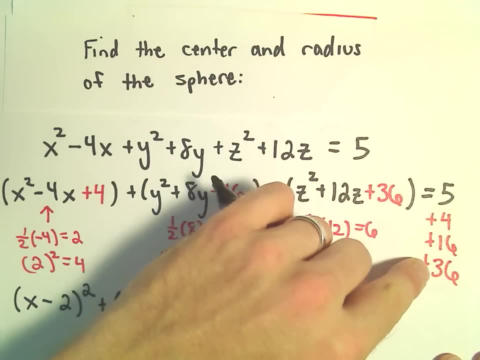 z squared plus 12z plus 36, we can write that as z plus 6 squared On the right side. if we add everything up, let's see. I guess we've got 20 and 36,, that's 56..